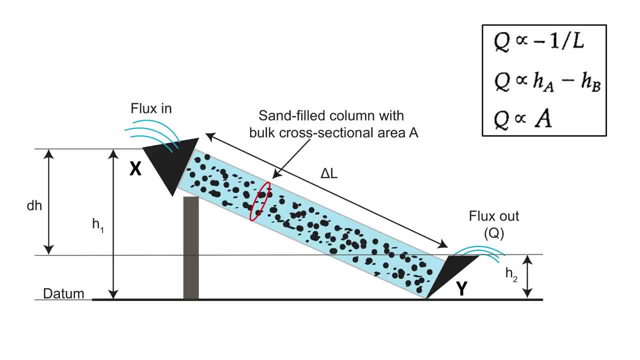 experiment he studied the movement of water through a porous medium. So here in the setup you can see that there is a cylindrical pipe and it has a cross sectional area of A, And this cylindrical pipe is filled with sand- porous sand- and the water is allowed. 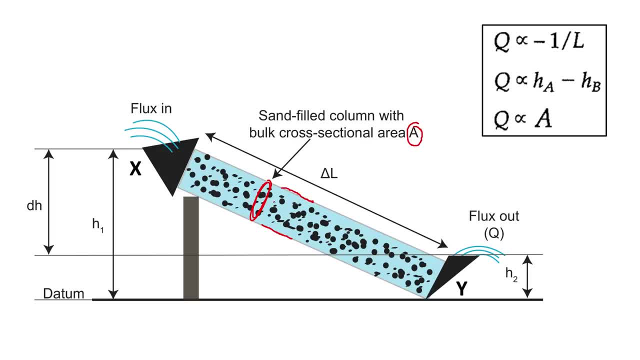 to flow inside it. So you can see this point X where the water is going in and the point Y where the water is going out. So actually this water is going in at length. So this water is going out at location X and out at location Y because the energy of water 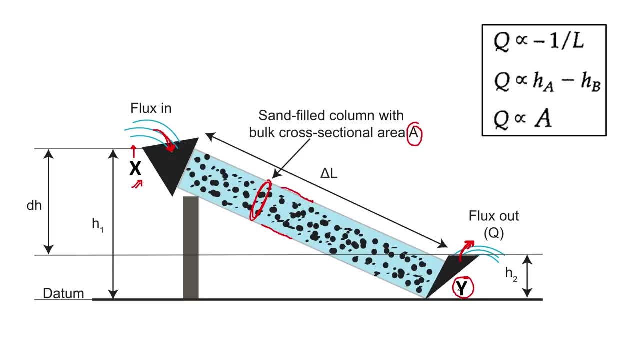 at X is higher than the energy of water at location Y. So this energy here is called the hydraulic head, or pressure head, Or simply you can call it head. So this head at this point X is H1 and at point Y is H2.. This is the height. So this 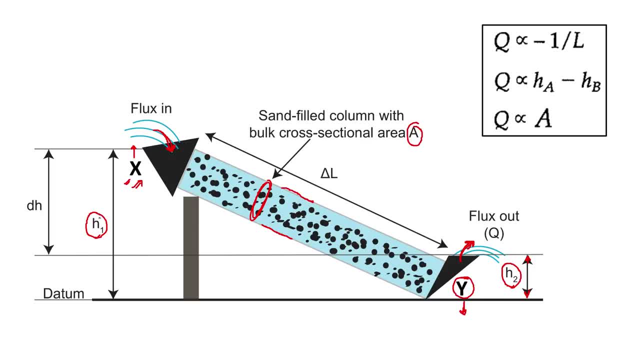 energy of water is written here in terms of height of water, That is, in the unit of length, And this unit of length has come from Energy per unit area. I mean, sorry, weight Energy per unit weight. So this energy, at this point it is the total mechanical energy, That is the which includes the kinetic energy. 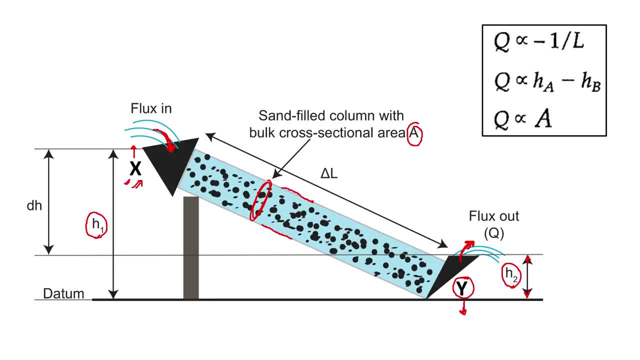 gravitational potential energy and the energy of the fluid pressure. So this is the total energy. Hey, This is represented in terms of the unit of length, which is the head. By doing energy per unit weight, This experiment, you can see that This is the height. 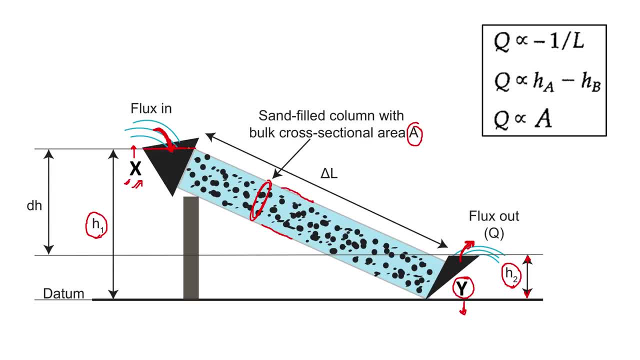 Of the water in the cylinder. Okay, But it has covered Somealer Power. So this is the edge when height of the head, one husband, except This head at location Y. okay, but suppose if I open this I insert a vertical pipe inside the stopper. 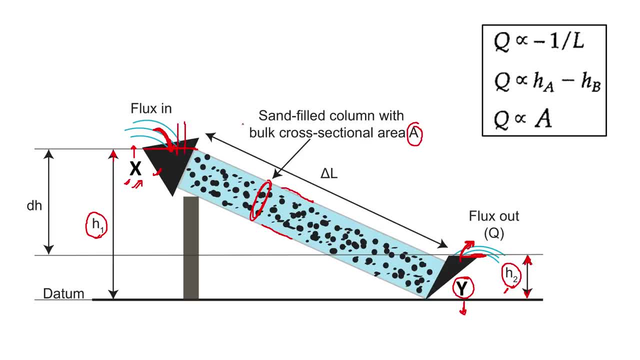 okay, it's like a stopper and a vertical pipe is inserted inside. okay, so what happens is that the water would try to flow in this pipe. okay, upwards if it is under some pressure. okay, that is, if the energy is high. okay, as I told you, the total mechanical energy. so the water will try to go. 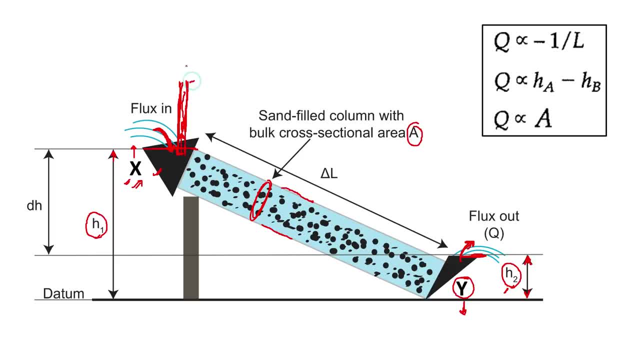 inside this pipe which is open at the other end. no pressure is applied from here, only it is the atmospheric pressure. okay, so the water will move inside and it will attain some height. okay, suppose at this point. okay, so, if, if I do this, this would be the head at location X. okay, the? 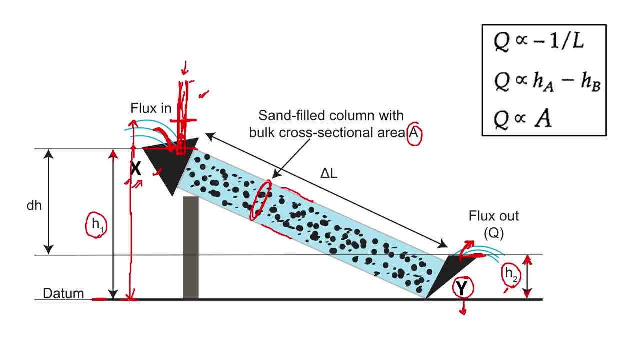 height is measured from a common datum? okay, from where you will measure this? the other head? okay, at the same, at the same point, okay, so, uh, in this case, where it is written H1, it might have been just here. I mean, the water wouldn't go up. okay, even if the pipe is inserted, the water level is till here only. okay, it can be. 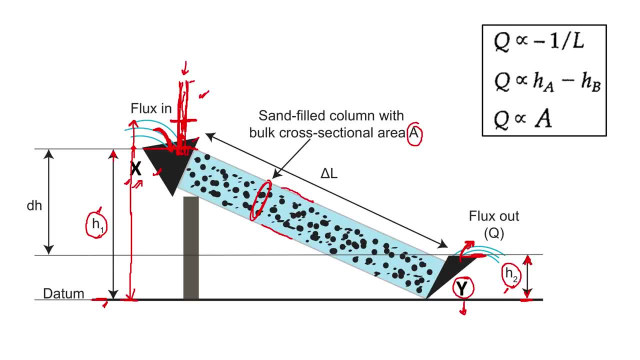 at any level, depending upon that, upon the head. okay, the energy of water. okay, so suppose I mean you can think like this water could even go in the opposite direction, right? I mean, if you apply some force right, apply some pressure from this Y point, okay, right, you can imagine that. right. so you put a lot of pressure in the water flow starts to flow. 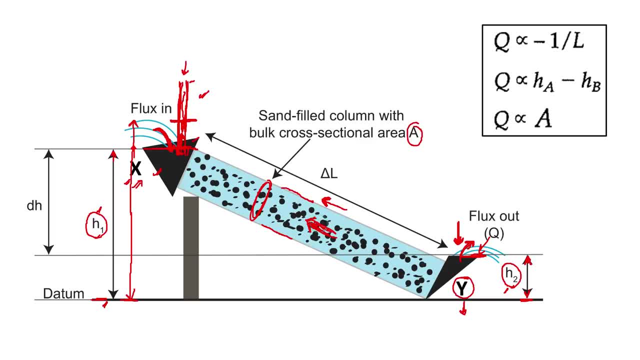 in the opposite direction. okay, so how will you measure the head now? okay, now you will say that yes, this is the H1, because the water is still at this point and here the water is at this point and in the Darcy law we have seen that the water flows from a higher head to a lower head. 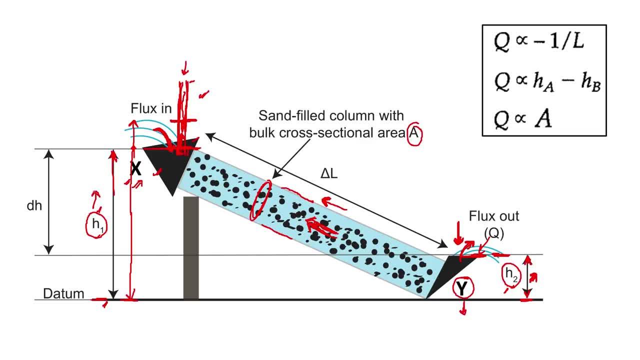 okay. so if this H1 is high, is has a higher value, the water will flow. flow from X to Y, okay, from a higher energy towards a lower energy or lower head. but now, if the water is flowing in in this direction and you're applying pressure from this, 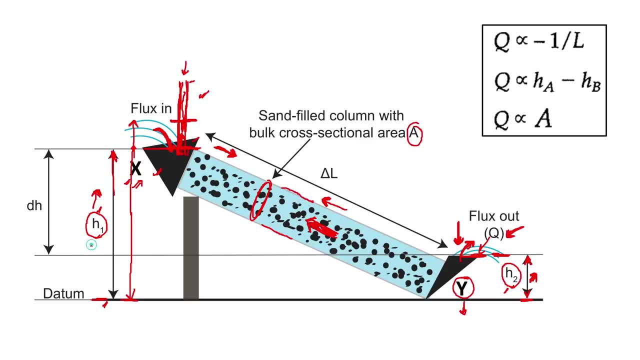 direction by the height of this head or the head. simply, head is has a higher value, right? but even the water is flowing in the opposite direction. how can you measure the head now? okay, so this we cannot see by this point, where there, from where the water is coming out, right? 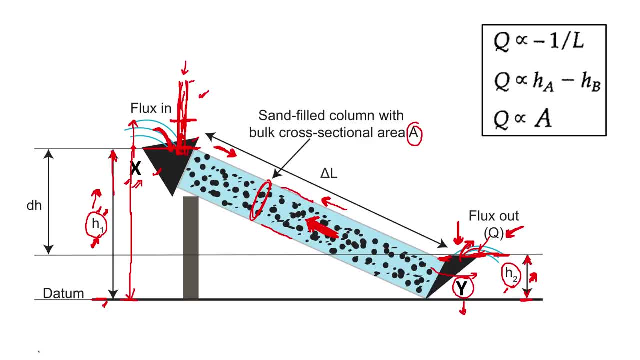 this, uh, this head, at this point now, when we are applying a lot of pressure. okay, there is some point. okay, we'll do that with the help of the vertical pipe. okay, now we have inserted a pipe here. okay, the water is allowed to flow inside this pipe. 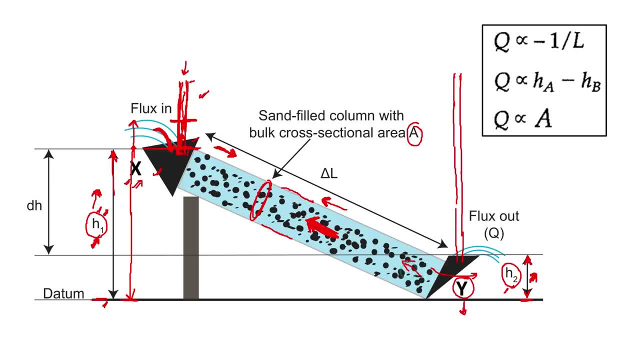 okay and nowhere else. okay, it is, either the water is going in this direction or in this pipe. okay, so the water at this point would be somewhere, would rise somewhere till this height, or maybe higher, but higher than this head. okay, okay, anywhere. I mean this. I give the example previously, but now maybe the height is still. 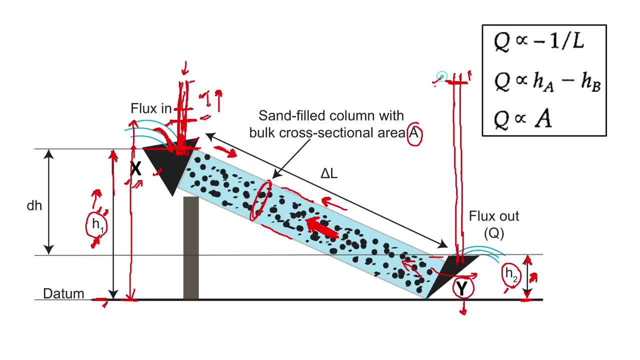 here, but it has to be lower than this head. okay, because the water is flowing in that direction. okay, and this water is flowing in that direction because the head at point Y is more than the head at point X. okay, so this is the way of measuring the actual head. 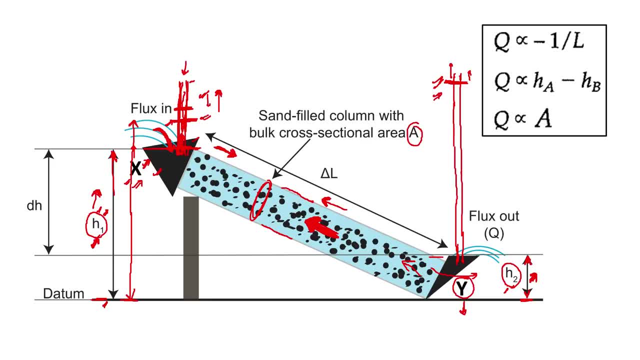 okay, and the length between the head. this is the length. it is represented by capital L? okay, and it is important in case of Darcy law when we will discuss the formula, so I'll erase all this. okay. so in this setup we can see that the L? okay, or the difference. in the length, or? or you can say it'll be different depending on the attitude of the board when we are trying to carry the steeper board or— L� can be a little difficult, but you can make all that sense. as i was saying earlier, It's easier if you think that you cannot do a very perfect workout software. so you should consider doing one of those three functions that are relevant to the way it will work. 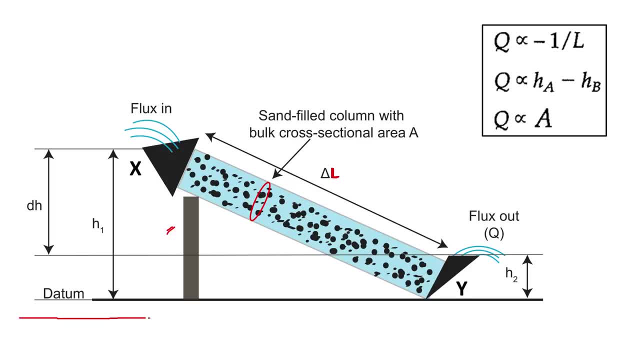 So you can say that this from this point- suppose A, this head is- may be 100 meters and from here, so from point A to this head, it may be around 300. so this is 100 meters and this is so this length, this total length till point Y is 300 and till point X is 100 meters. So this is the 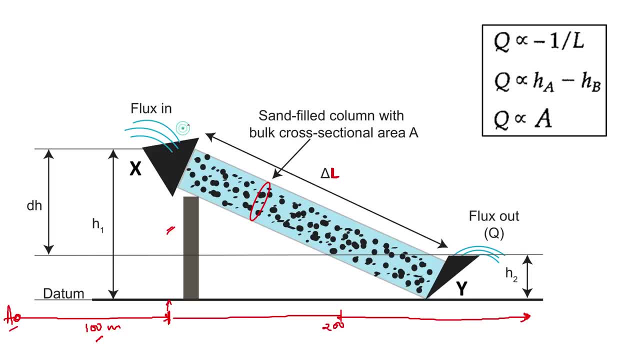 difference between the length at Y and at X and at Y, So it would be 100, 300 minus 100, which will be 200.. But here we will not take the horizontal distance, So we have to take this distance actually. So maybe it is somewhere around. 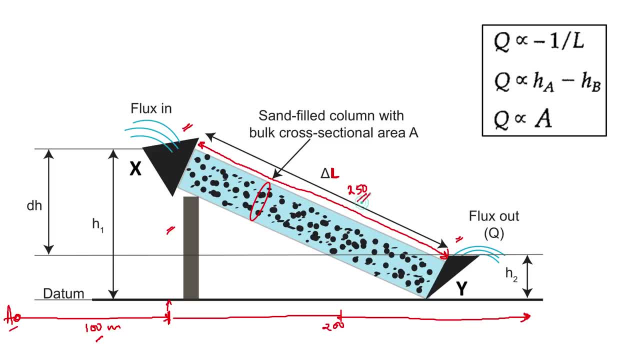 250.. So now Darcy found out that through his experiment he said that the discharge- This is the discharge Q, capital Q is also called the volumetric flow rate, Or simply the volume of water. So this is the volumetric flow rate. 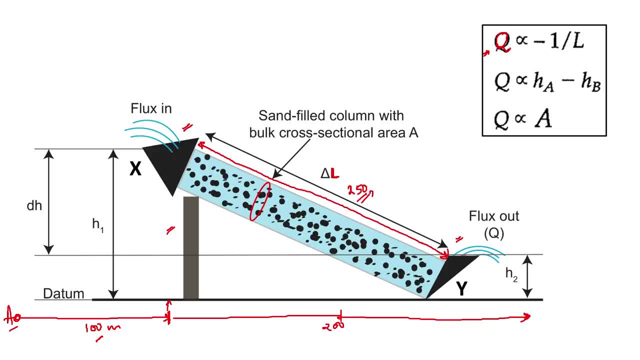 So this is the volumetric flow rate. So this is the volumetric flow rate, This volume of water coming, water coming out from this point that just flux out per unit time, That is the volume of water flowing out per unit time. So this, this volume of water. 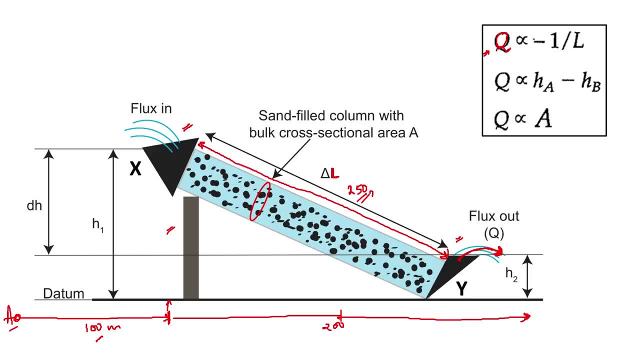 which is flowing out is inversely proportional to the length l, and this Q is directly proportional to the head difference. So the more the difference between this H1 and H2.. h1 and h2 more will be the discharge, and this discharge is directly proportional to the area. 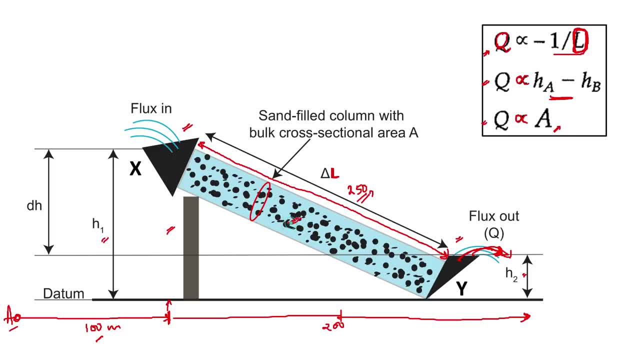 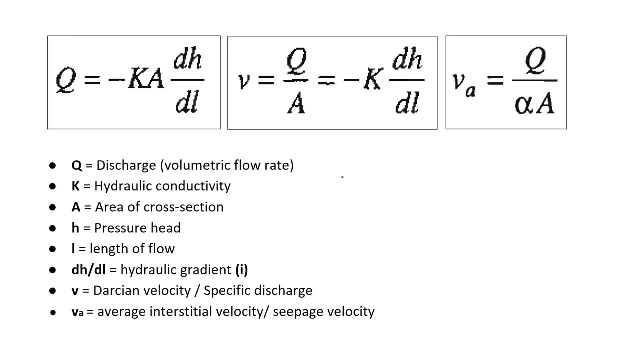 of cross section of this cylindrical pipe. so the more the area, the more will be the discharge. now, as you remove the proportionality sign, you get a constant which is k. so this k is called the hydraulic conductivity- okay. or it is called coefficient of permeability- okay, it is not same as permeability. it is coefficient of permeability- okay, we'll. 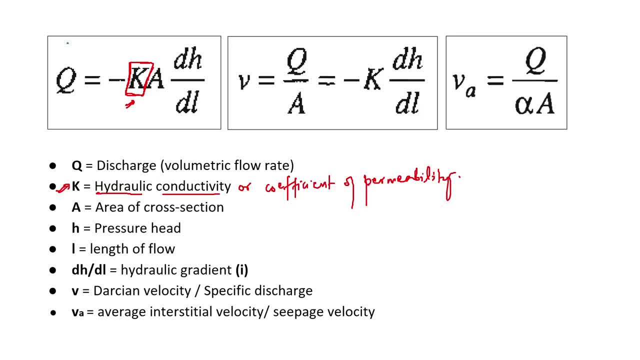 see the difference soon. so the formula becomes what. okay, so the formula becomes what. okay, so the formula becomes what. q is equals to minus k hydraulic conductivity into a, which is the area of the cross section, into the difference between the head and the length between the two. 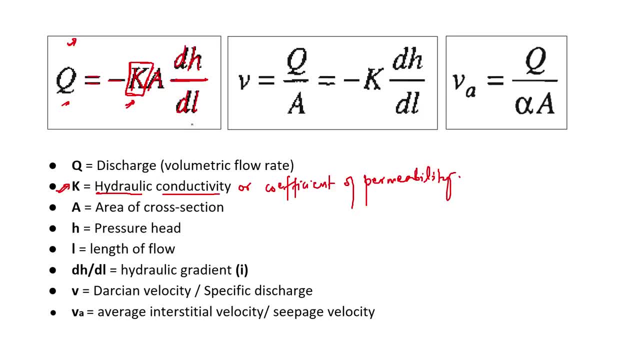 points which we are, i mean, considering. so this goes on to this. v, which is q, upon point. q is equal to one a, so it is volumetric flow rate divided by the area of cross section. so what you get is the unit of meters per second, which is the velocity. so this is the velocity of 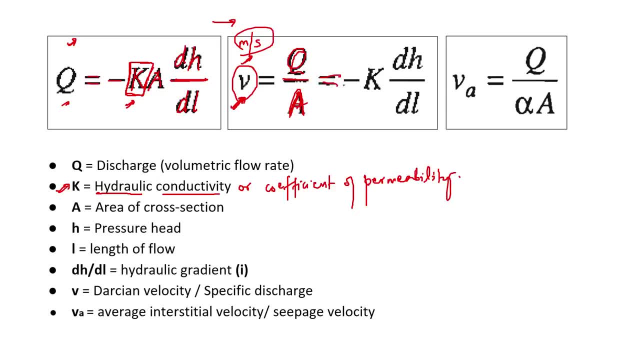 water at point y in the diagram. okay, so v becomes what it is: k, dh by d, l. so, simply, area goes here and we get v, which is called the darsen velocity- okay, darcy, darsen velocity. or it is also called the specific discharge- okay, specific discharge. so the units of this meter of water per second flowing out. 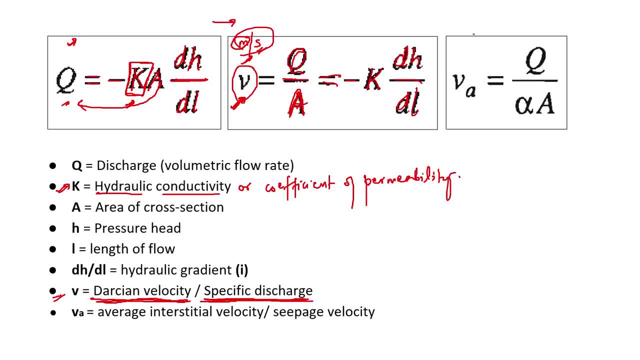 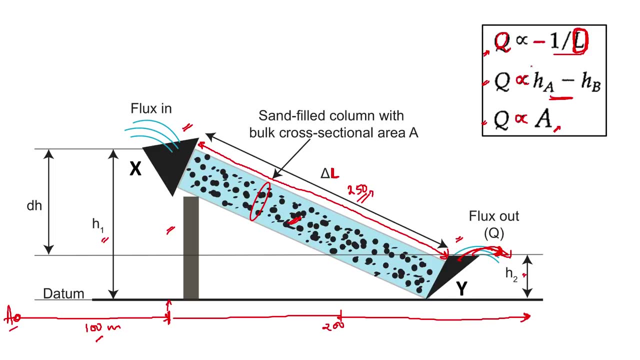 now, why the minus? and we'll discuss this formula in some time. okay, why the minus sign here? we'll discuss that. okay, so previously in this slide we have seen that there is a minus sign here and because of this, we we are getting a minus sign in the whole formula, right? so suppose? 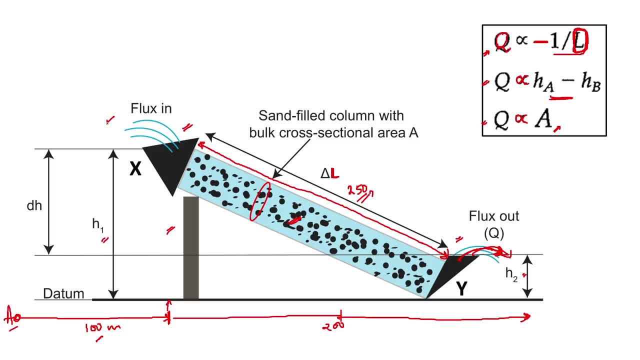 if you are subtracting, if you are subtracting h1 minus h2, which is h minus h1 minus h2, will give you a positive value, right, because h1 is greater than h2. so in that case you have to subtract the length at this point, the distance from a at this point, with that of 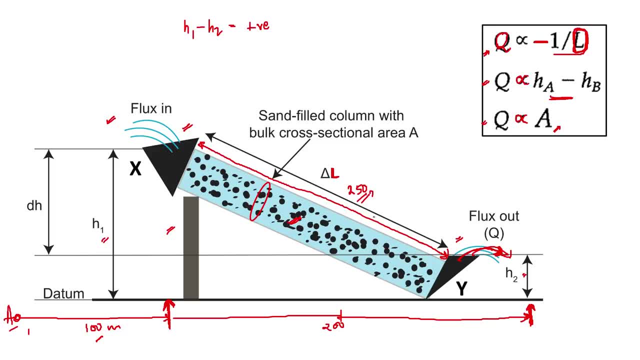 point y. okay, so what you have to do here is is 100 minus 300. you have to do right. so what you will get is minus 200 meters. so now you can get right that why there is a minus sign. okay, and even if you maybe you suppose, uh, like, uh, the water is flowing from uh x to y, so this has. 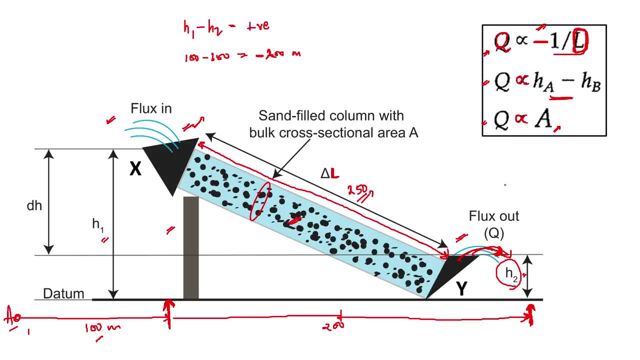 to be the final h2, okay, and now we'll, uh, do that final minus initial thing, okay, so it would be h2 minus h1, okay, and this would be a negative value. but now we have to do what, the similar thing we'll do here, that we will subtract 300 from 100, so you, so we'll do that, so we'll do that, so we'll do that. 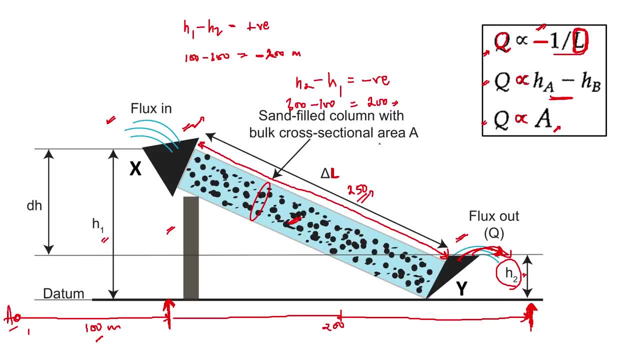 we'll not get a minus value here, we'll get 200, okay. so i let me tell you again the length is this. okay, i'm just considering it 200, but the actual length is here. okay, it might be around 250, maybe something we have to apply some hypotenuse, okay, i mean this trigonometry, okay, 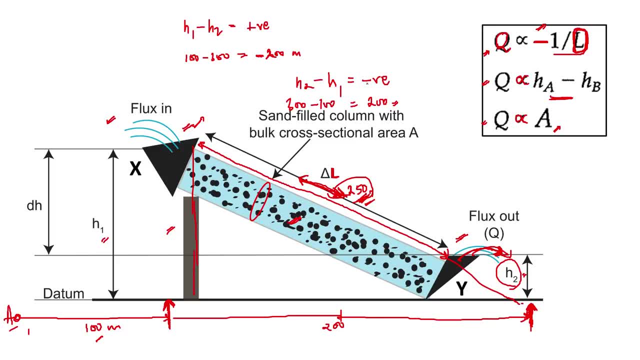 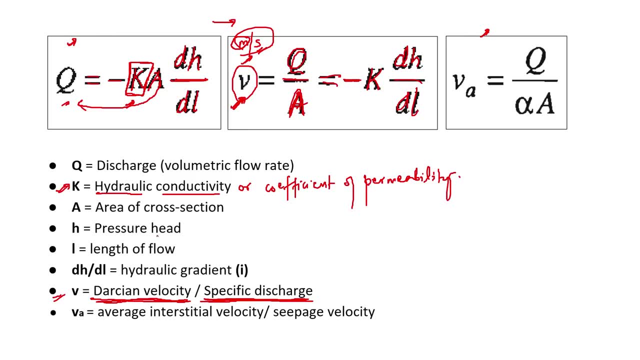 so, so we'll get a minus sign anywhere, okay, so, basically, this, uh, this term, okay, this term, which is dh by dl, has to be negative. okay, and therefore a minus sign here. and this, this whole term, is denoted as small. i, okay, this is called the hydraulic gradient. okay, this is the gradient. 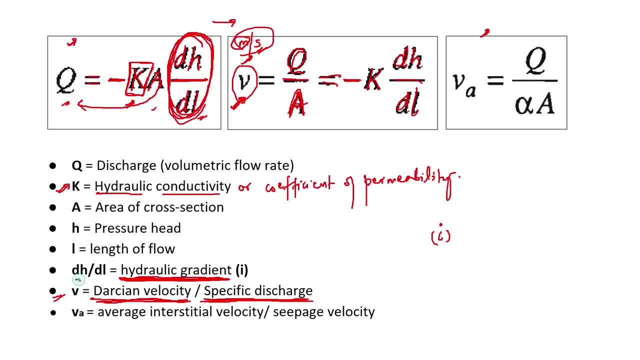 which is height, difference in height upon difference in length. okay, this is denoted by letter small i. okay. so i mean you don't have to just consider the minus sign. whatever you answer you will get, you will get it in positive value, okay. so, no, no worries about i mean, you have to consider the minus sign. 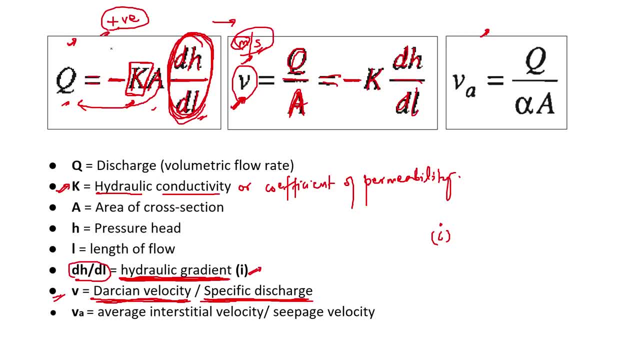 or something. okay, just just remember that the answer would be a positive value. okay, so, because nothing here is negative. so now let's see what is hydraulic conductivity? it is simply the ability of the material to transmit a fluid and, in case of hydrogeology, it is the ability of the aquifer to 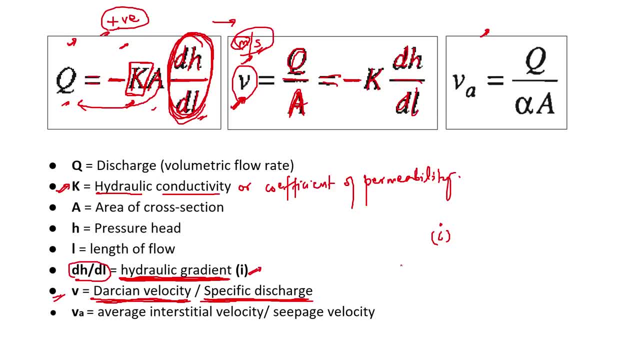 transmit water. okay, the unit of hydraulic conductivity is meters per second, which is same as darsen velocity and or specific discharge, and hydraulic conductivity is the property of both the fluid and the medium, that is, both the aquifer and the water which is flowing through it. okay, so 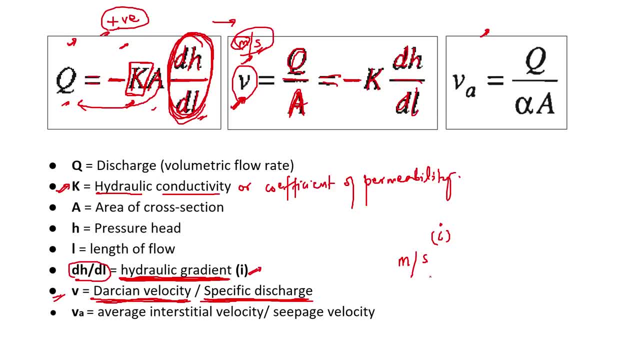 you could imagine, this will begin to flow through it for about f一个 video very soon and this means that if you allow oil, which is more, more viscous fluid, if you allow it to pass through that aquifer, the hydraulic conductivity will change. okay, and if you allow water to flow through another aquifer, of different property and of maybe another medium, the hydraulic conductivity will still change. and if both fluid and medium is changed, you can imagine this becomes flexible. so when you sunlight, the water flows in, while your fluid will be through. and if both fluids are också, because they are completely different dla water, so you will see thatolic conductivity will still change. 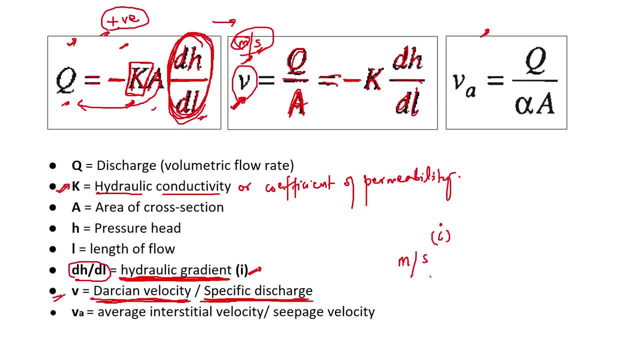 and if both fluids and media measures change. so that's where we are gonna mean that of the same thing. if it results well, if you allow some στο match Arizona, at least some or two捏 kinkwk so that that awakens- the hydrolic conductivity will still change. and if both fluids and media measures are passing fruit, the hydraulic conductivity will change for the hear voice protectors. 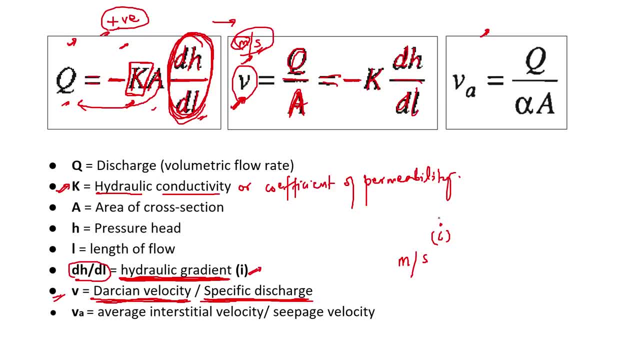 is changed, then obviously it will change. i said earlier that it is not permeability. okay, it is coefficient of permeability. so don't confuse it with simple permeability, because permeability is the ability of only the medium. okay, again with the same example, i will explain that. 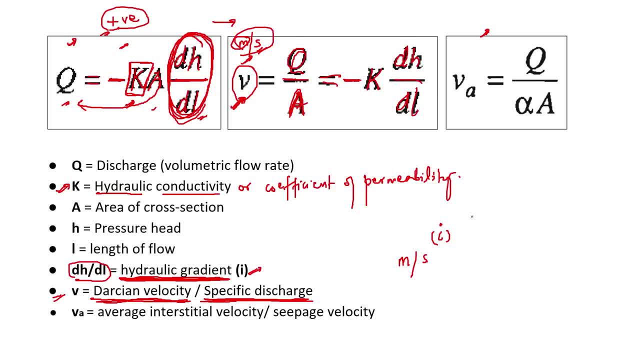 if you allow water to flow through an aquifer, it will have a particular value of its permeability. but if you allow oil to flow through that same aquifer, even then the permeability will be same because the medium is not changed and it is only dependent upon that medium and the unit of 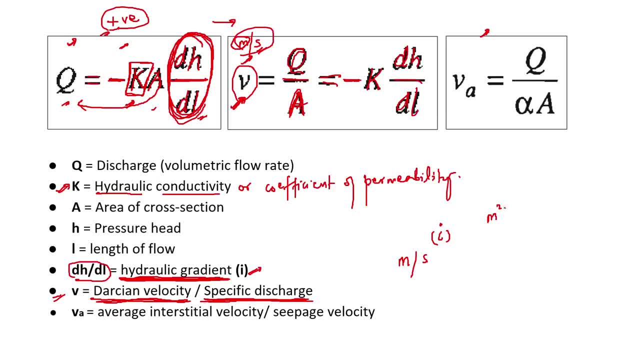 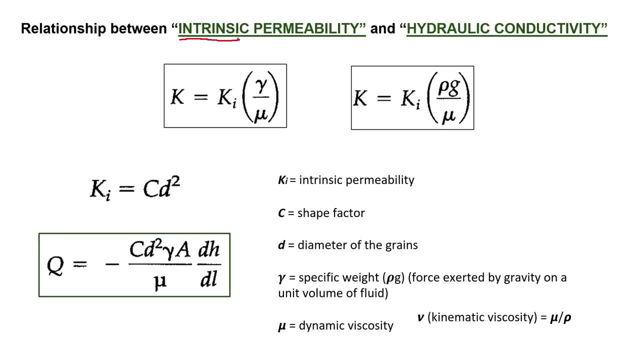 permeability is meter square, so let's see the relation. okay, simple permeability is called, also called as intrinsic permeability. intrinsic, you can say that it is maybe the internal property of it, so this is what we call intrinsic permeability. okay, this is also called intrinsic. 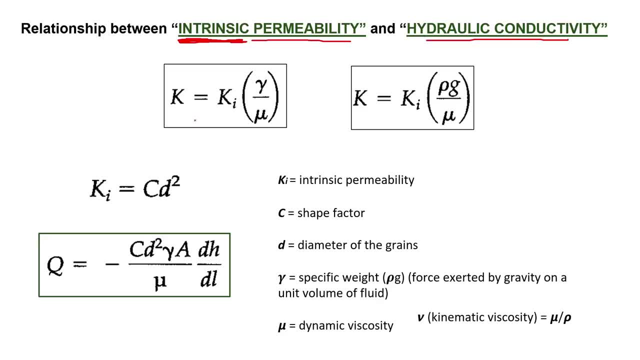 permeability- okay, this is also called intrinsic permeability- okay, this is also called intrinsic- of that medium, okay, and hydraulic conductivity. so this is the relation between intrinsic permeability and hydraulic conductivity. so you see that this is the specific weight of water, okay, gamma and mu is the dynamic viscosity of the fluid, okay, so you see that this hydraulic 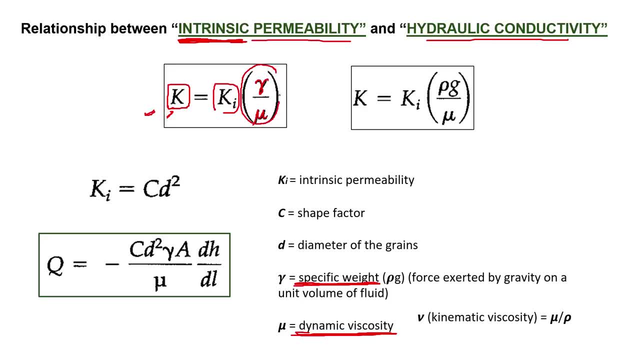 conductivity includes the property of the fluid. okay, or you can write it as: k equals to ki, which is Rho G upon mu. okay, so this specific weight is equals to Rho G. okay, specific weight is the force exerted by gravity on a unit volume of fluid and, simple. this intrinsic permeability is dependent only. 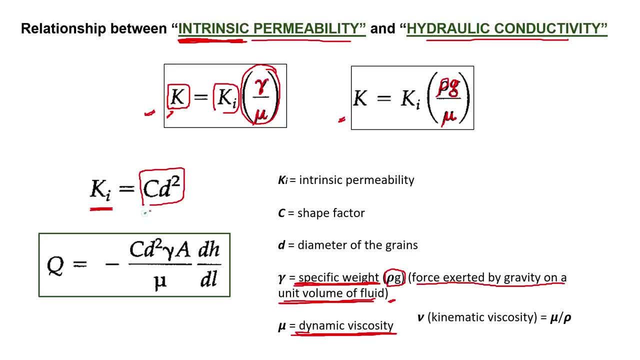 on the medium. so formula is CD square, which is: C is the shape factor and D is the diameter of the grains. so it is proportional to the square of the diameter of the grains. okay, so basically it is: ki is directly proportional to the d square, that is, the square of the diameter of the grains. 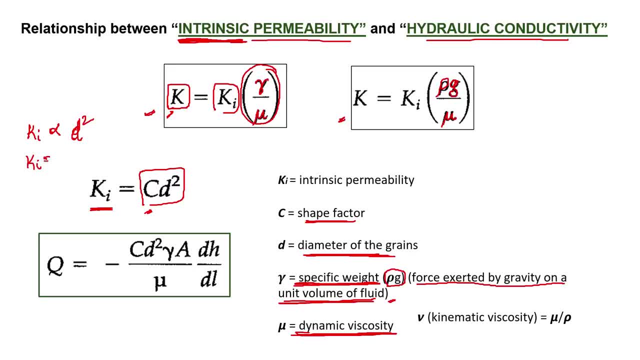 and there comes a constant, which is when you remove the proportionality sign, which is c, also called the shape factor. okay, so the probability depends upon the diameter of the grains, which will decide the porosity, and the shape, which will decide the permeability, and vice versa also. 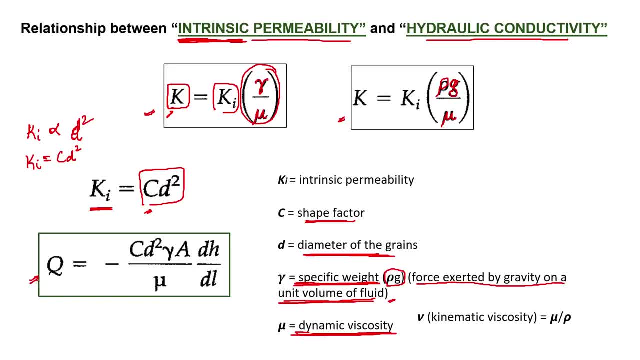 so you can write this specific discharge as this formula. okay, so you're putting cd square here in place of ki, and then it is gamma specific weight upon mu. okay, so this becomes this formula. okay, so remember this also. this is also really important. and there is one more term, which is kinematic viscosity, which is mu- i mean nu- and it is equals to. 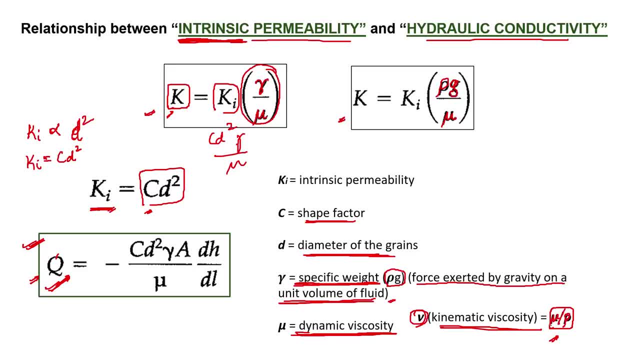 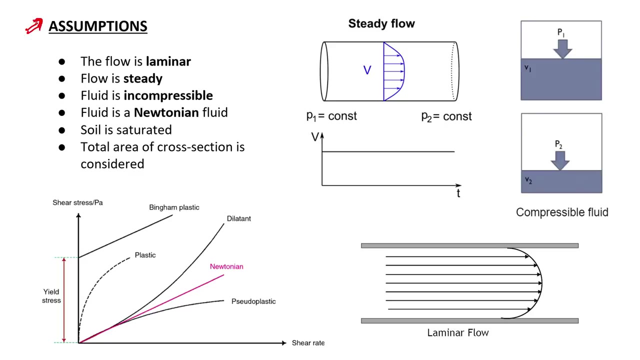 dynamic viscosity upon the density of the fluid. i hope all the formulas are clear to you because these are very important for both gate net, student and jam. also, ninety percent- i'm sure that there would be a question from nazilo. so let's see that, what assumptions we have taken to apply this law. okay, because 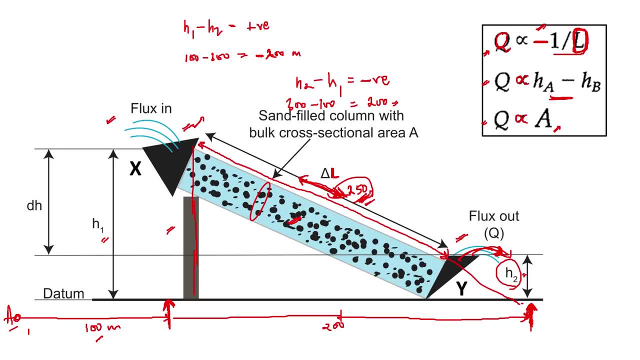 this condition which we have seen in this experiment. this condition is not same as the real scenario which is in the aquifers right. the aquifer is not a cylindrical pipe, the area of cross section is not this cross section, but this voyager motion here goes forward and then, if you, 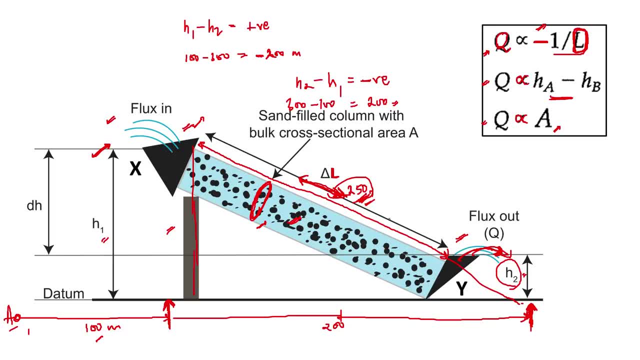 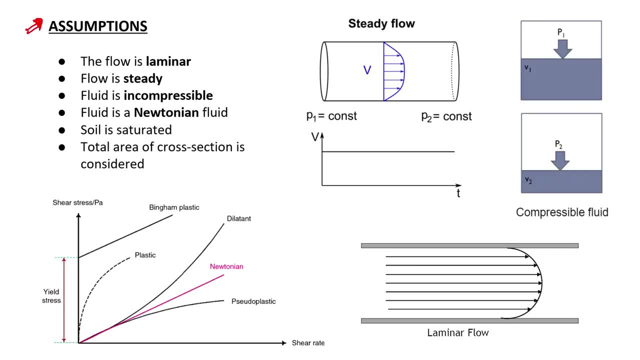 cross sectional area. We are not considering the whole cross section, So we will see the assumptions. So first assumption is that the flow is laminar. Laminar flow is like this: There is no haphazard flow of water, It is flowing in a single line straight, No rapids. 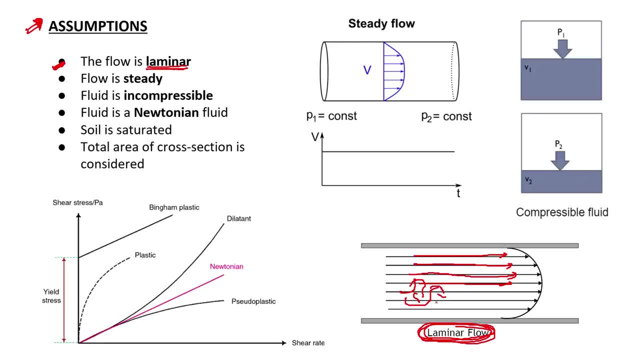 no hair in the movement of water, which you see sometimes when the velocity of water is high enough. So this is the assumption that the flow should be laminar. It is measured by the quantity of water, The quantity which is the Reynolds number. The formula is rho Vd by mu, And if the Reynolds 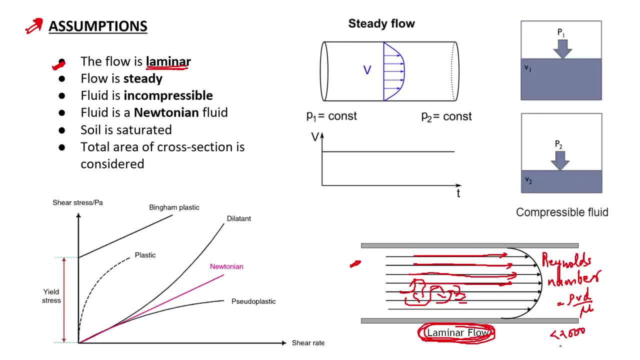 number is less than 2000,. this means that the flow is laminar, So it is valid for only laminar flow. Second is that the flow is steady. The flow should be steady. That means, if you see this graph, this is the steady flow. If you see this graph, you see that with time, the velocity 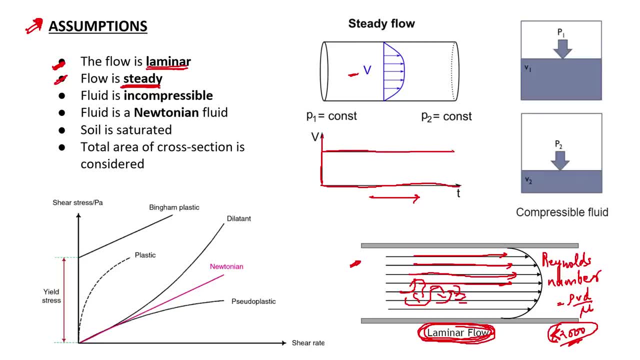 of the water is not changing. That means here also the velocity of water is same. And as the area is not changing, the velocity of the water is not changing. So this is the Torah all the time, because the discharge will also be the same At this point of time. 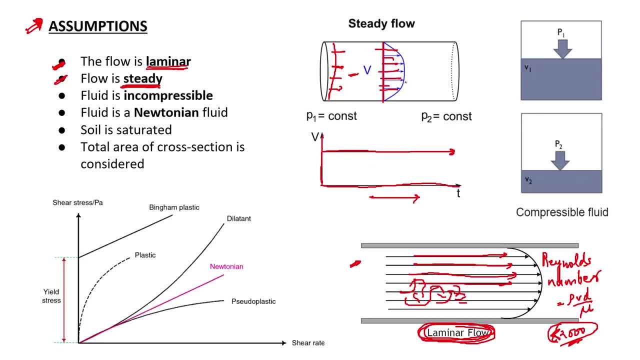 at this place at a different time, the velocity will be same, The discharge will be same and from here also it will be same. So this should be the condition for applying Darcy's Law. Next is that the fluid is incompressible. The fluid is incompressible means that the 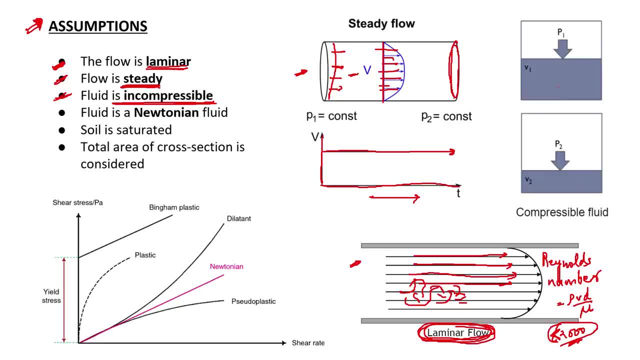 fluid. the density of the, the density of the fluid should not change with pressure, Why? Because there is a decrease in pressure or There is a gentle pressure. The fluid is inexpressible pressure. So this we can see, that it is simply incompressible and this one is a compressible. 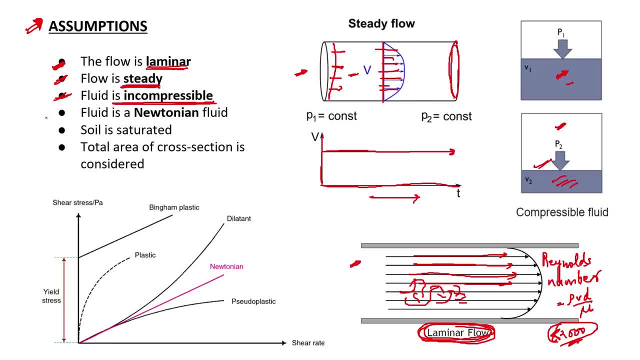 fluid. Fourth, we can see that fluid is a Newtonian fluid. So the fluid should be a Newtonian fluid, which says that there should be no change in the viscosity of the fluid with stress. On applying stress, there should be no change in the fluid viscosity. So this: 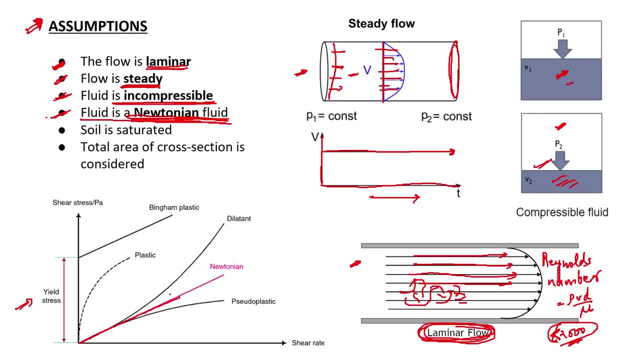 is the graph. Again, this is the Newtonian fluid, So it is the applied stress and it is the shear rate. Again, you can see all these different materials having different property, But here only newtonian fluid should be there, or we can assume it as the newtonian fluid you want to. 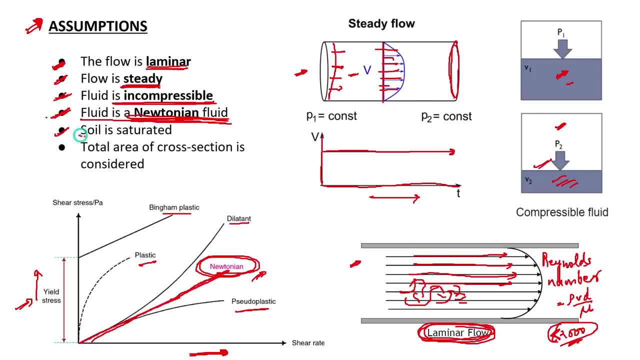 apply this formula. next thing is that the soil is saturated. okay, that means the whole, uh, the whole pipe, the whole cylindrical pipe or the whole aquifer should be filled with water. okay, should completely fill that volume, that in the, in the- let me show you the diagram- and in this whole, 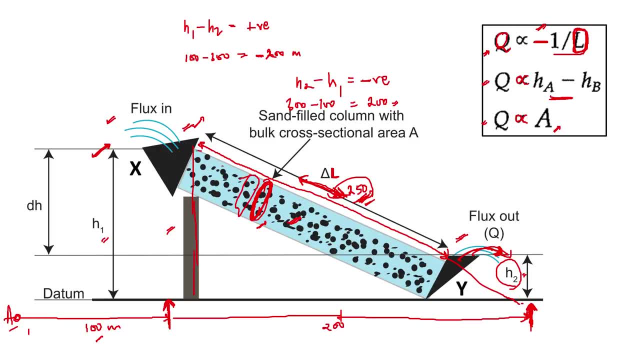 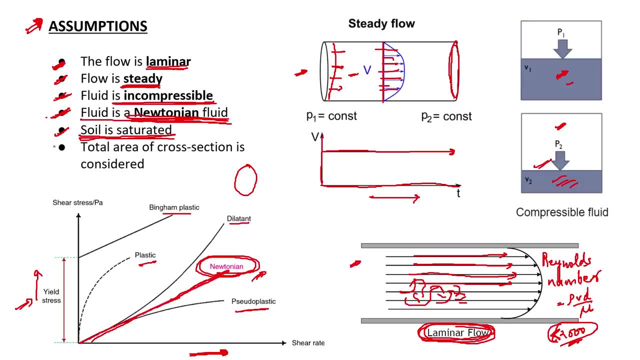 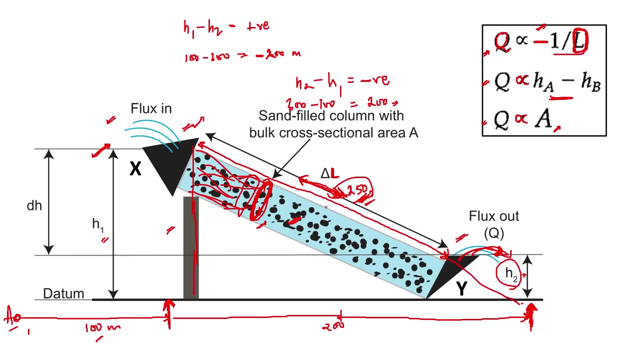 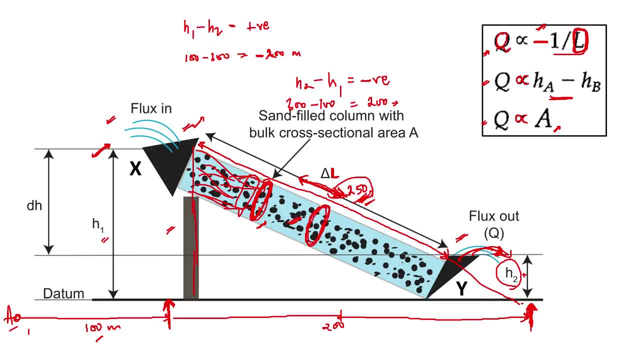 is taken. okay, so that means that this area we are putting here is, it is the complete area of cross section, right, so the water can be maybe here- okay, as i did here- and would be flowing around here, but we are even. then we are considering the whole cross section and without considering the 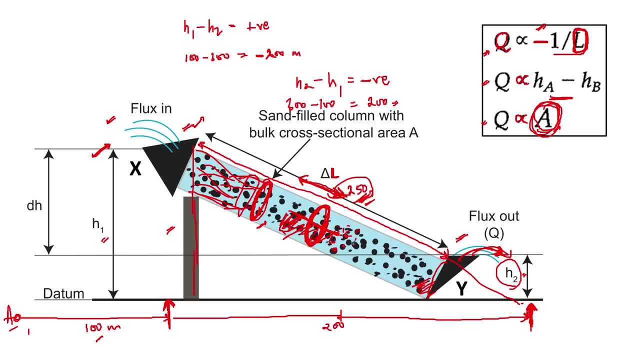 whole cross section and without considering the whole cross section and without considering the whole cross section, this sediments, okay, because we already know that the water is coming from the pores, right. okay, it's traveling inside the pores, the connected pores, okay. so we should not consider the complete. 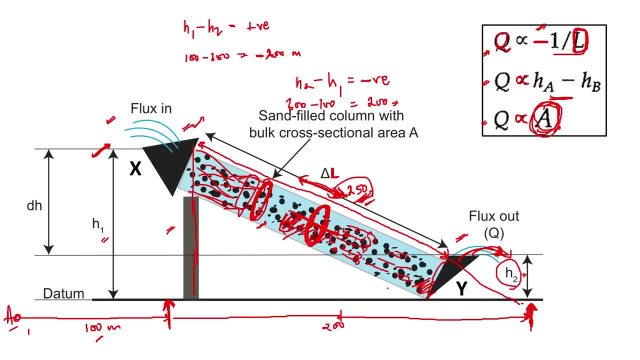 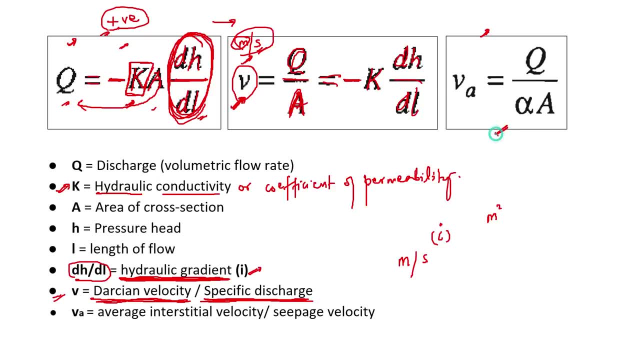 area of cross section. but we consider here- but for that we have a solution, that is this formula. okay, so i told you i'll discuss it in the next video. okay, so i told you- i'll discuss it in the next video later- that this uh, uh we. 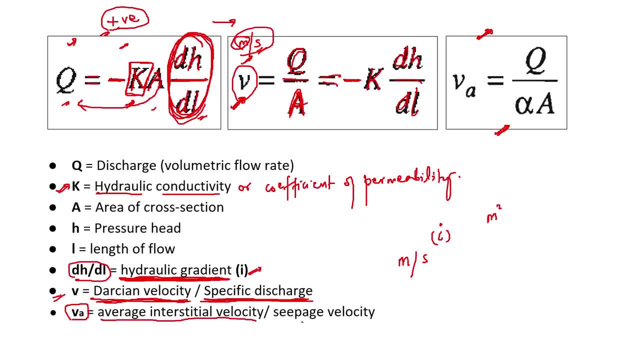 a is the average interstitial velocity, okay, or the seepage velocity, okay, so this is simply v, which is divided by alpha. okay, this Q by A is divided by alpha, okay. and as the porosity will always be impacted by alpha less than one, okay, you don't have to take it in percentage, okay, otherwise, otherwise it will be. 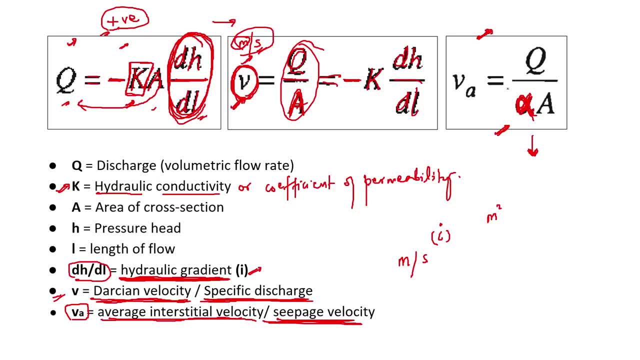 more than one, but it should be less than one, okay, so if it is less than one, this va will always be higher than v. okay, right? so, uh, i mean, you can understand that simply that the discharge is same. right, the discharge is same because here also it is q and here also it is q. 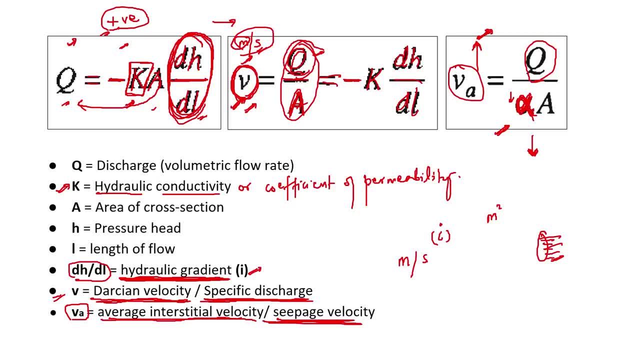 for the same discharge in the same time. okay, it charges the volume per unit time, right, so the velocity has to increase. right for having the same discharge, because the area is reducing, because we are dividing it by the porosity, or you can say that it is better to say that it is the effective porosity. 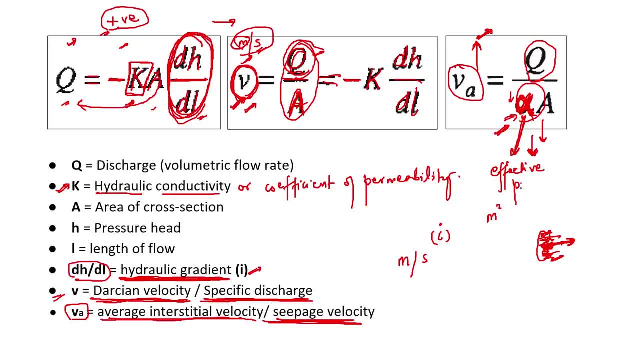 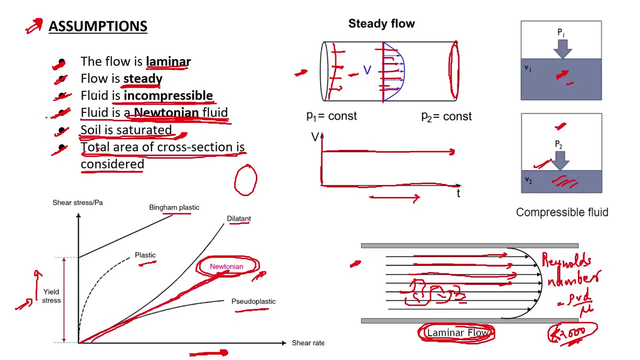 because the water will flow through the connected pores. okay, so the volume of the connected pores divided by the total volume is the effective porosity. okay, not the porosity. okay, so these are all the assumptions which we take, but the assumptions are also taken as such that it does not change the answer very much. okay, so, in in our case, 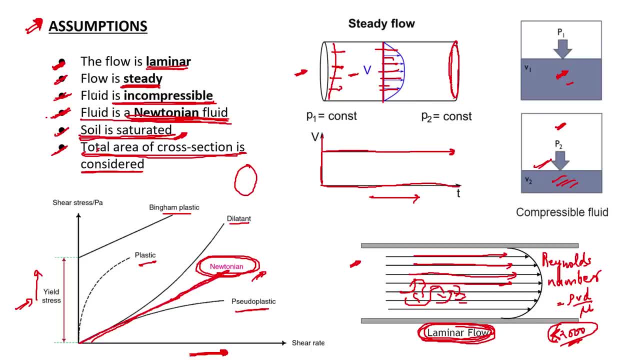 that is the aquifer and water system. the flow is laminar. yes, it is more or less laminar because the water flows at a very, very, very low speed. okay, it is in terms of meters per day, okay, so it is very slow and that is why the velocity. 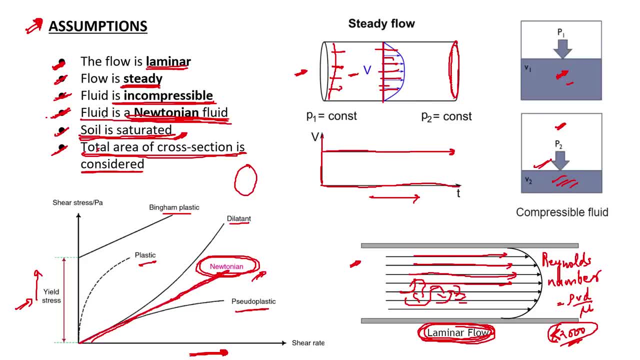 is very less and the flow is mostly laminar and the the fluid is incompressible. yes, the water, water is almost incompressible and the fluid is no Newtonian. and, yes, water is Newtonian. so we can easily apply this assumption. the soil is saturated, it might be, it might not be, and the total area of 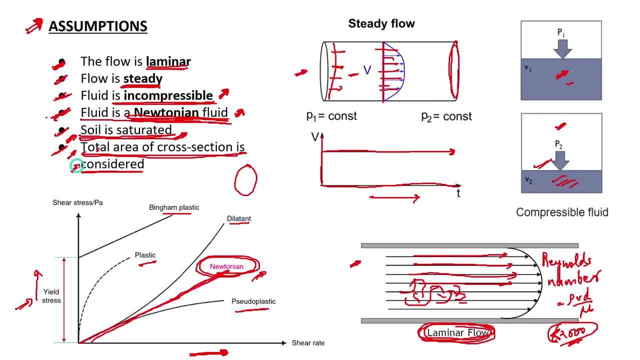 cross-section is considered okay. so these might be same but might be different. but it will not affect the answer very much, but there are some differences, the real differences which for which we apply a different formula. so, like, like, you can say that there is another assumption, that the flow is a 1d flow only means that 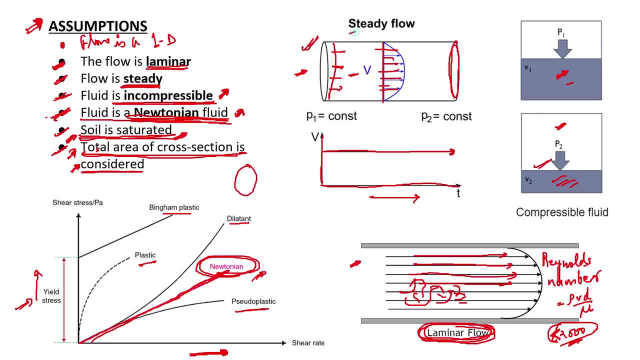 through this pipe. this pipe, the water is flowing in this direction only. okay, straight straight out of this pipe. but this is not the actual case, that in the actual scenario in the aquifer the water is flowing like this: up and down, left and right. okay, it is flowing in all the directions. so later the GATE students. 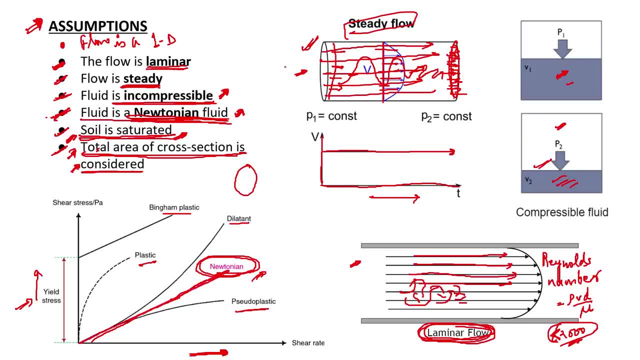 would definitely study about the flow equations, which is, which might be 2d flow and might be 3d flow and in this case, in the case of Darcy law, we have seen the 1d flow okay and the flow is not steady. so we see the equations as the steady flow equation and 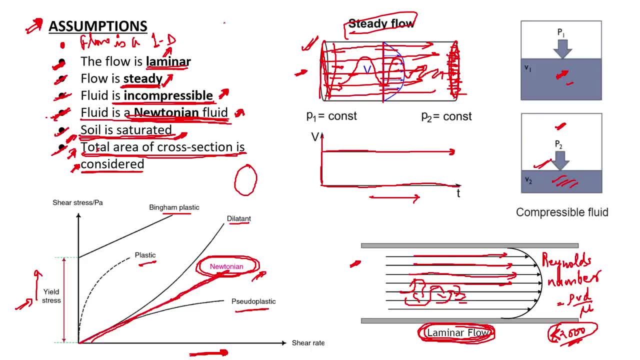 unsteady flow equation. okay, so this is all. you will study later. many of you might have studied already. so this is all about the darcy law and i try to teach you as conceptually as possible. so you might be having a lot of questions. so for that you can ask, ask in the comments. we'll reply.